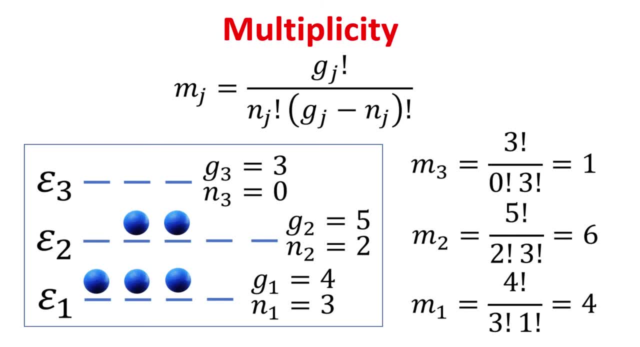 by the combination formula, which is g factorial divided by n factorial and divided by g minus n factorial. You can find the link to the video on permutations and combinations in the description below. Using this formula, we can easily work out the multiplicity for each energy level for: 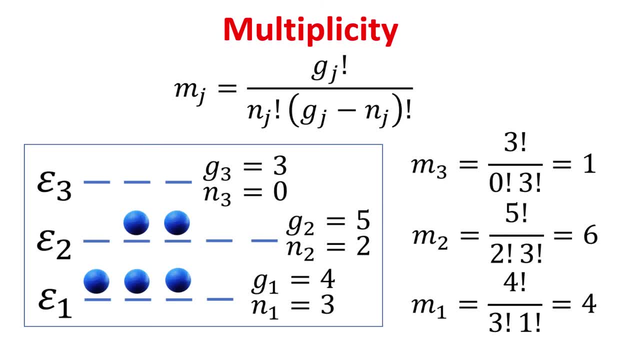 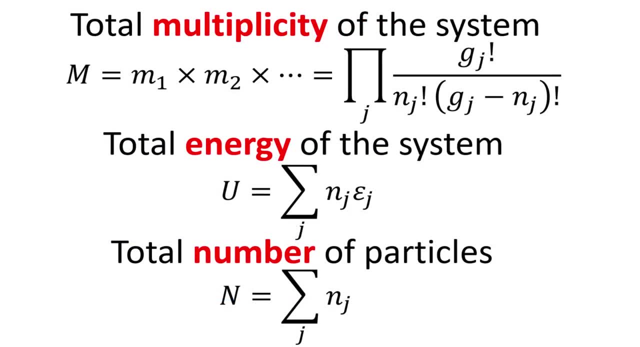 the system on the left, with the particular distributions of electrons: n1 equals 3, n2 equals 2 and n3 equals 0. The total multiplicity m of the system would then be the product of the individual multiplicity of all the energy levels. The total energy of the system, u, would be the 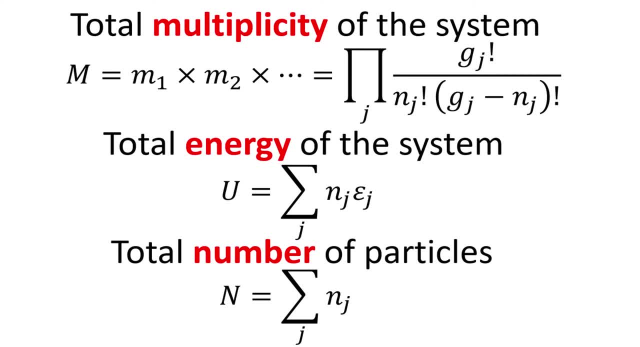 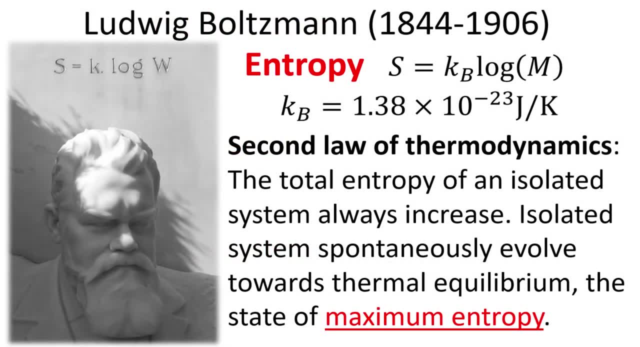 product of the energy and the number of electrons at that energy level summed over all energy levels. Lastly, the total number of electrons is constrained to be n. In order for us to proceed to the next step, we need to first borrow an equation from Ludwig Boltzmann's tombstone. 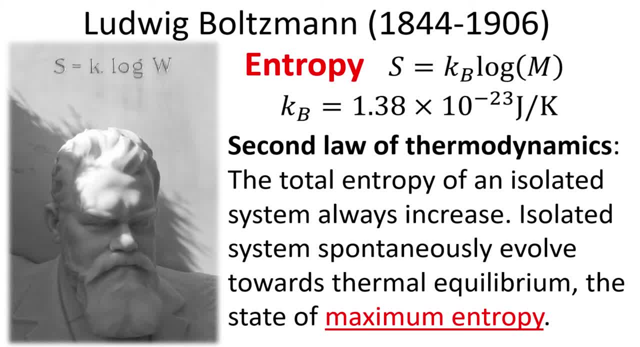 Here the entropy s has a definition in terms of the number of microstates, given by k sub b, the Boltzmann constant multiplied by the natural log of the system, multiplicity m. An important insight by Boltzmann into the second law of thermodynamics is the realization that 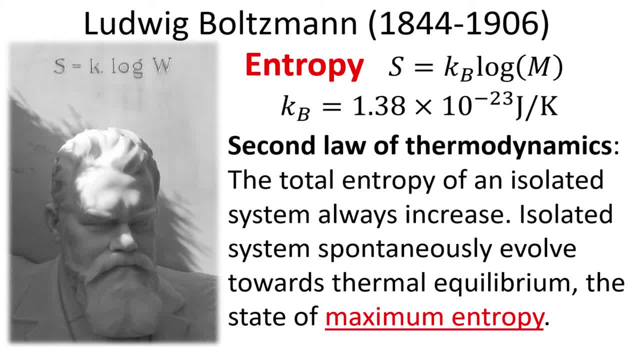 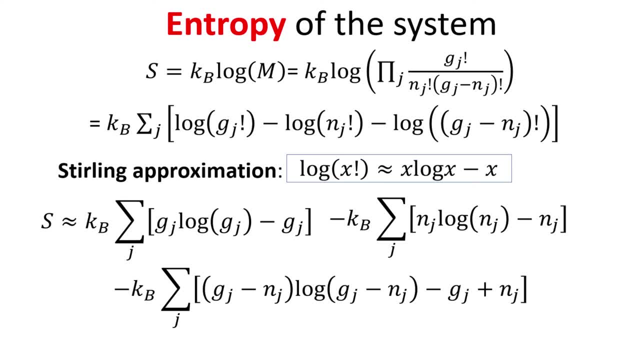 isolated systems spontaneously evolve towards thermal equilibrium, the state of maximum entropy. Let's work out the entropy of the system using the Boltzmann definition of entropy. We substitute the multiplicity expression into the logarithm, which then allows us to write the product of the multiplicity of the different energy levels as a sum of logarithms. Next, 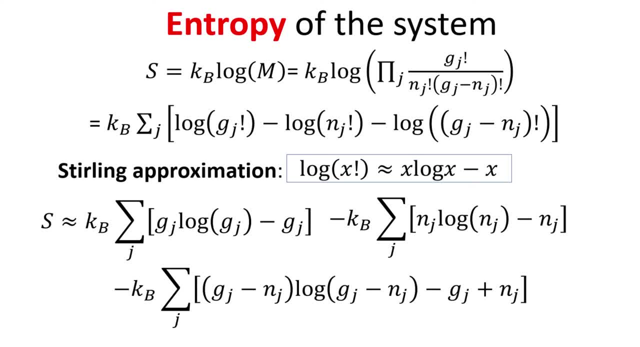 we recall the Stirling approximation, as shown, which, in the limit of large x, allows us to write it in a form without the factorial Applying. the Stirling approximation then allows us to arrive at an expression for the entropy without any factorials. This will serve to be very expedient. 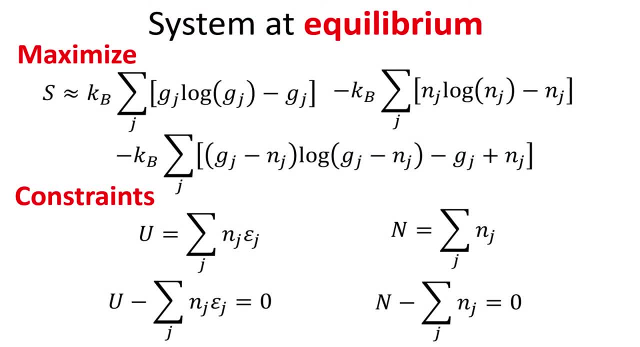 in our next steps of the derivation. Next, taking the Q from Boltzmann, to find the electron's distribution at equilibrium, we should seek to maximize the system entropy while at the same time imposing the constraints on the total energy and the number of electrons. To solve this trio of equations, we shall resort: 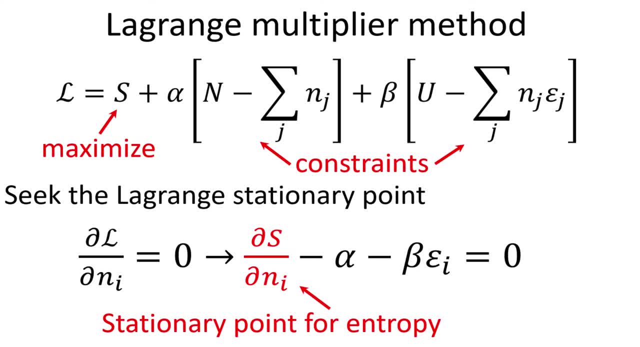 to the method of Lagrange multipliers. The method of Lagrange multipliers is a strategy for finding the local maxima and minima of a function subject to equality constraints. We introduce an auxiliary function, L, which consists of the entropy s which we seek to maximize. 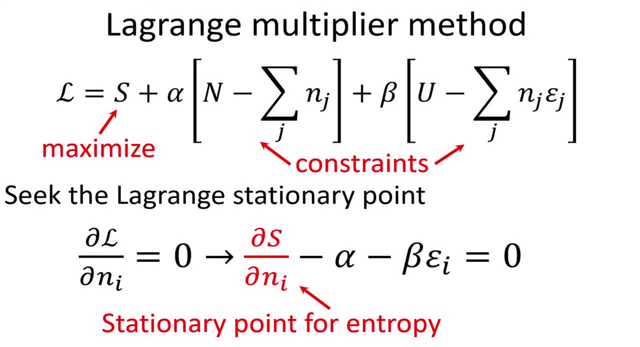 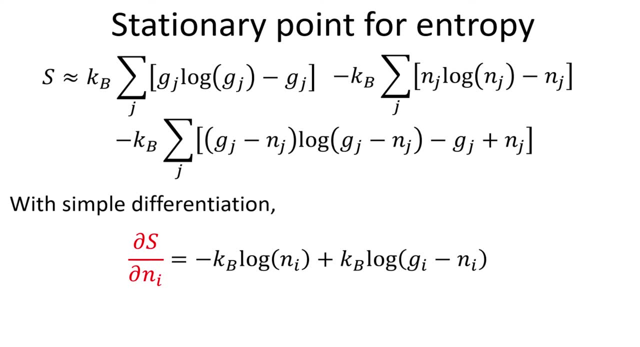 We seek to find the Lagrange stationary point with respect to the number of particles at each energy level. i. To proceed, we first have to find the stationary point for the entropy s Recall, the entropy expression we derived earlier. with Stirling approximation, We can work out the stationary point for the entropy by taking differentiation with respect. 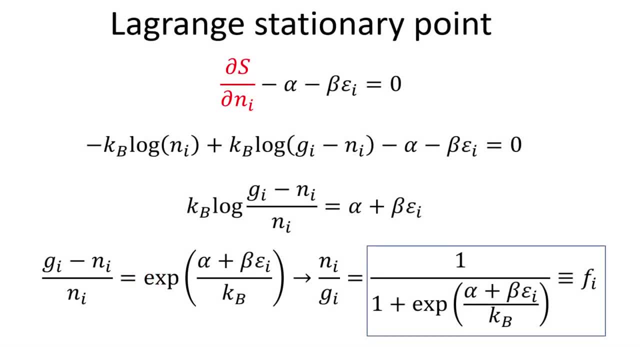 to n, sub i. Returning back to the Lagrange stationary point, we can now substitute the entropy stationary point into the expression. The terms involving logarithms can be combined and with some algebra we can arrive at an expression for the electron occupation for 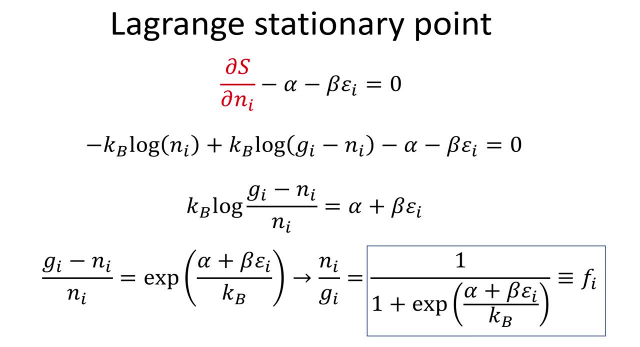 energy level i, which is the ratio between the number of electrons n sub i to the total available states, g sub i- at that energy level. This occupation factor is the Fermi-Dirac function we are after, and what is left is to determine the Lagrange multiplier constants alpha and beta. 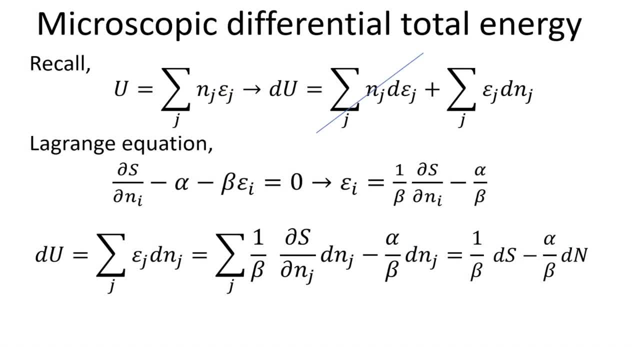 The way to determine the constants alpha and beta is to compare our microscopic expression of the total energy with that of the thermodynamic law. We begin with our microscopic definition of the total energy u in terms of its differential form, Since we are only interested in the 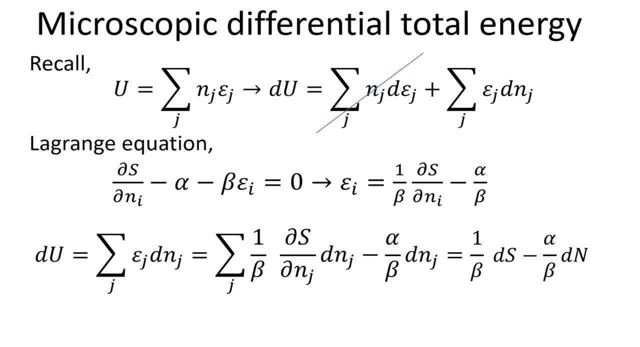 variation of n, we can eliminate the first term. We also recall our Lagrange multiplier equation and obtain an expression for the energy level. Substituting this into the differential of u expression, we obtained a new expression for the differential u in terms of the differential. 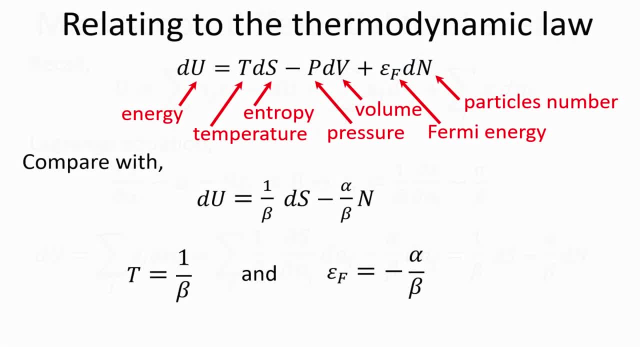 of entropy s and total particles number n, We recall the well-known thermodynamics law. A quick comparison to our microscopic expression of the total energy differential to the thermodynamic law allows us to relate temperature T to 1 over beta and the Fermi energy to the minus of alpha. 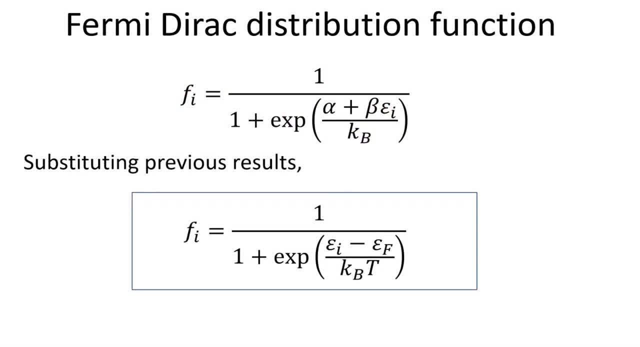 divided by beta. With this we can easily determine beta to be 1 over temperature T and alpha to be minus the Fermi energy divided by T. This then allows us to arrive at the final expression of the Fermi-Dirac distribution function. Stay tuned and subscribe, so you. 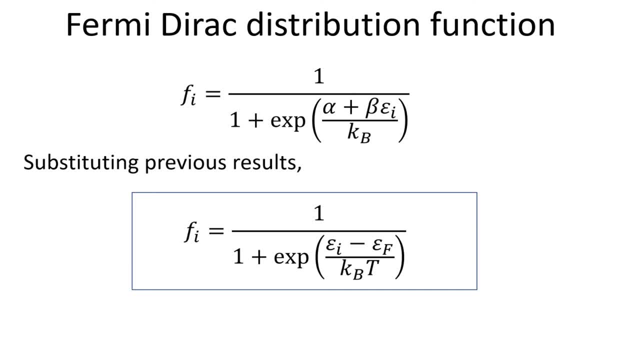 will be notified of our future episodes. Join our free Science Academy Discord channel to discuss science and technology. High school students are welcome to join and post your questions. we will answer them During our free time.